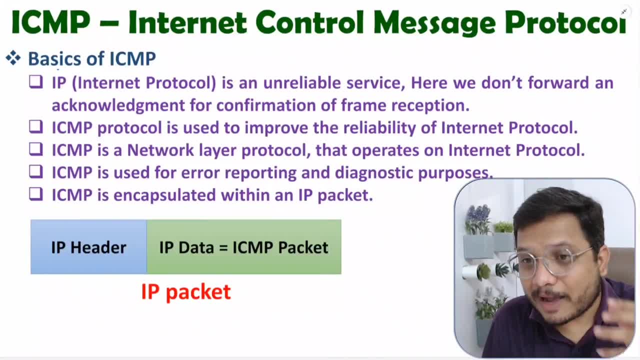 IP is unreliable service. why it is unreliable service? the reason is in internet protocol. in IP we don't forward acknowledgement. if you don't forward acknowledgement, then sender will never know whether frame is transmitted successfully or not. right, if sender is sending frame to receiver and if receiver is not giving acknowledgement, then how sender will come? 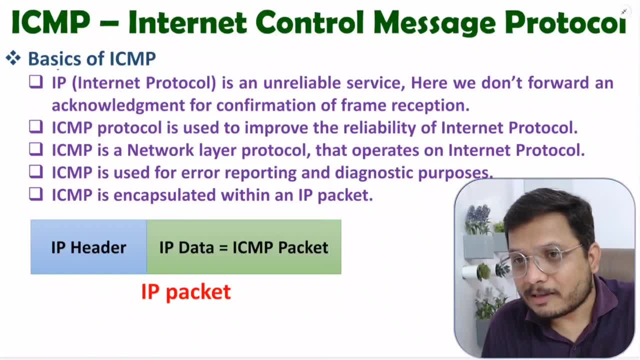 to know whether frame is transmitted successfully or not. that is not possible, right? so same thing is happening is with IP, with internet protocol, in that there is no acknowledgement and because of there is no acknowledgement, sender will never know whether frame is reached to destination successfully or not. and that is the point which makes IP unreliable. and to improve its reliability. 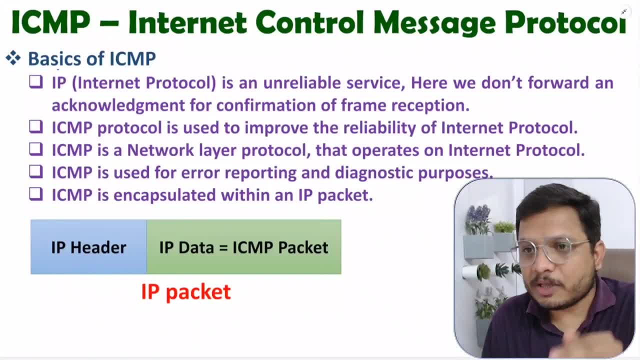 ICMP is implemented. see, with the use of ICMP we can say sender that this frame is lost somewhere in the medium as well as we can say sender that because of this reason, frame is lost in the medium. so, practically, ICMP is implemented on IP and ICMP is implemented to improve reliability. 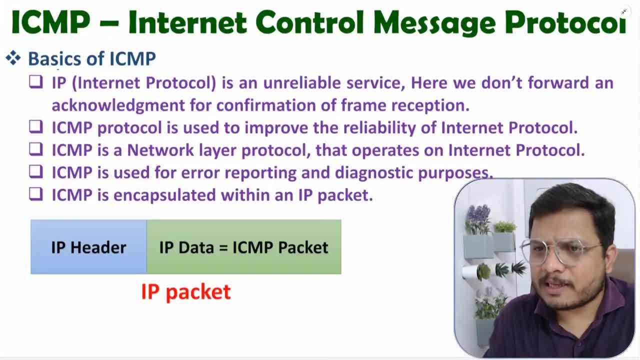 of IP, right? so let us see how many basics are there, then I'll explain you everything by practical examples. so the IP is unreliable service. here we don't forward an acknowledgement for confirmation of frame reception. ICMP protocol is used to improve reliability of internet protocol. ICMP is network layer protocol and that operates on internet. 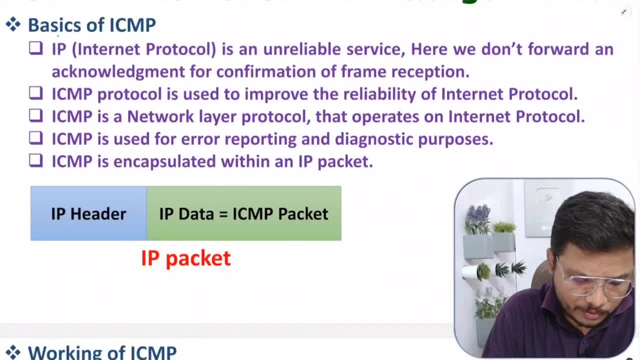 protocol. I'll show you how it operates on internet protocol see. ICMP is used for error reporting and diagnostic purposes. so in application part I'll explain you how it performs error reporting, as well as how we can have diagnostic of any computer network. I'll show you that practically right see. 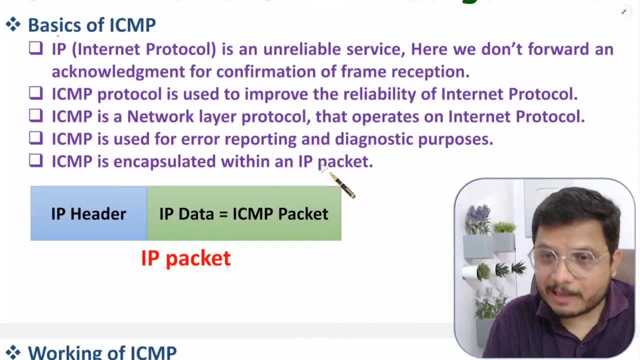 ICMP is encapsulated within an IP packet, like as if you talk about IP packet, then ICMP packet that is there inside IP packet. like you see, IP packet is having two parts: IP header and IP data. see ICMP packet. that is there in IP data, right? so ICMP packet that is encapsulated inside IP packet. that's why I'm. 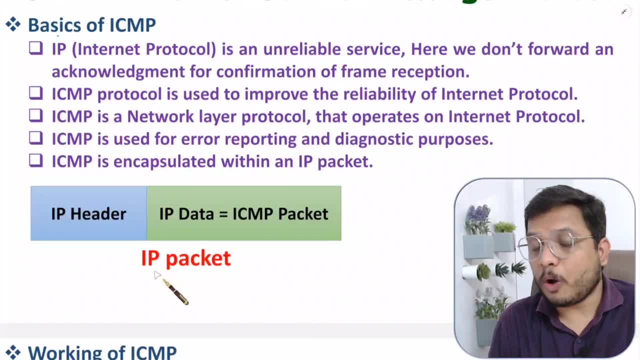 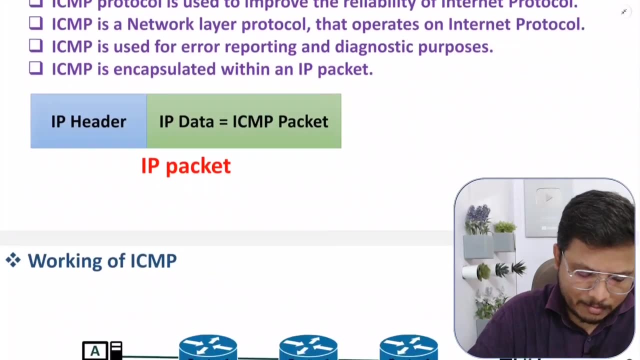 saying like: see ICMP, that is implemented on IP, and why we are implementing it. we want to improve reliability of data transmission using IP. so, as I have told you, there is always possibility, right? so let us try to understand that by practical working, so that will give you more clarity. so, before I, 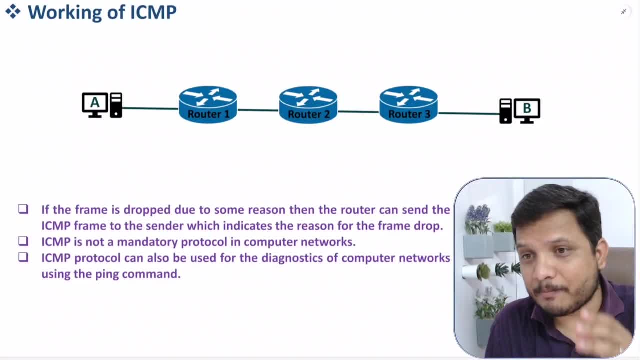 start with explanation of working, let me tell you: ICMP protocol, that is not compulsory protocol, right here. ICMP protocol, that is optional protocol. now let me explain you how ICMP protocol functions. for that, what I'll do is I'll take one example in which this host a wants to communicate with host B. 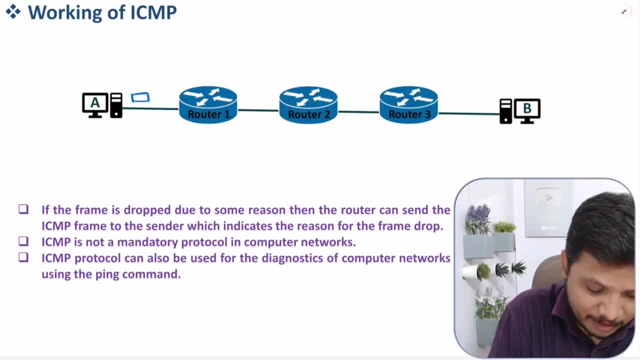 so here, let us say, host a is transmitting one frame over here towards host B, right, Right, Host A is sending frame to host B with addresses in this frame. So what will happen? This frame will be routed via router one, then it will go to router two, then it will. 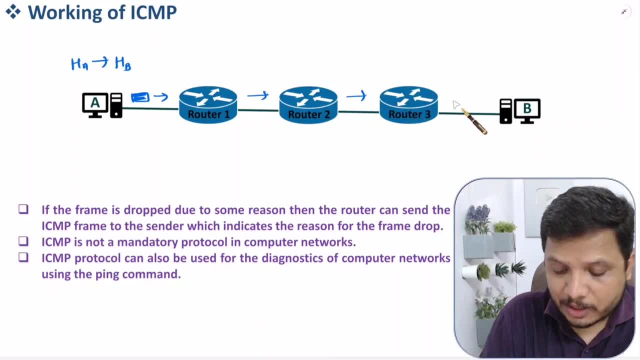 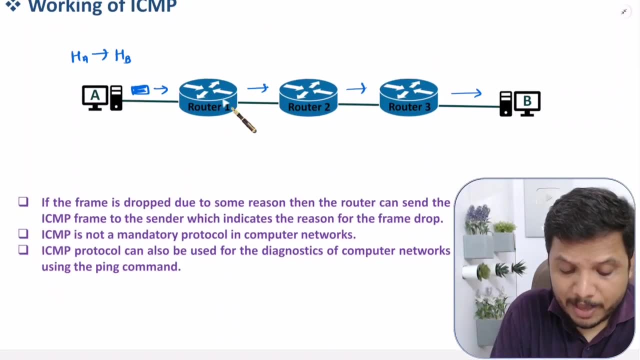 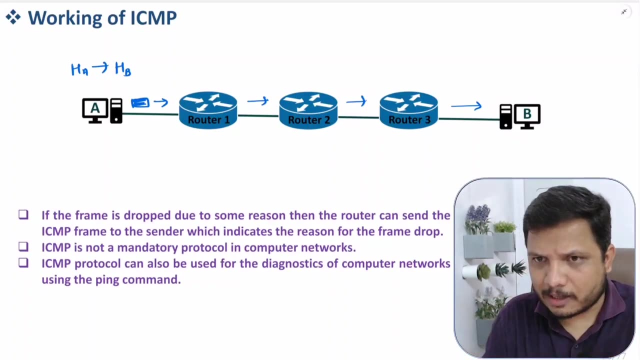 go to router three and then frame should reach over here to host B. But that is always possible that in this network frame may get lost somewhere. There can be many reasons, right? Let me tell you one basic reason. Like, let us say here, this router is so congested. 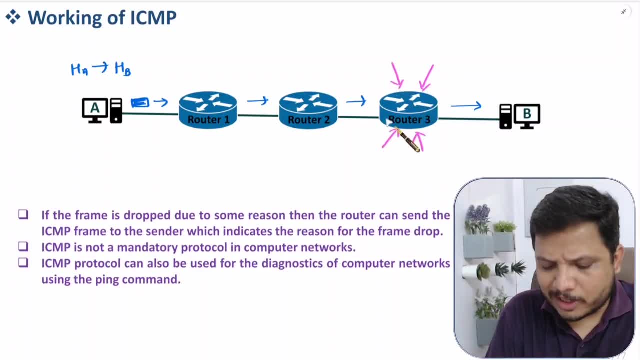 This router is so congested right. So much traffic is there on this router. There may be so many LANs connected over here with this router three. So because of that, as if I say, here frame loss is there, Here there is frame loss right. 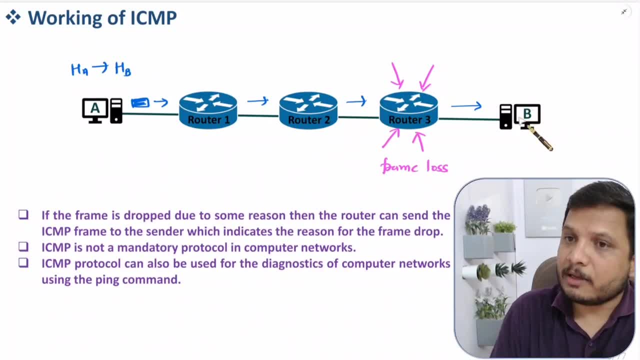 So what will happen? As per internet protocol, this host B will not get lost. It will not receive this frame. That's why I have told you IP internet protocol, that is unreliable service, But with the use of ICMP, with the use of ICMP, we can make it bit reliable. 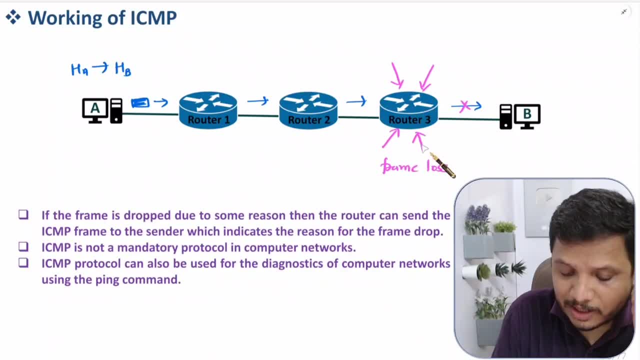 Now how See? as if router three is so congested, as if router three that is so congested it cannot forward a frame over here, Then what router three will do is router three will forward ICMP frame over here, ICMP And based on ICMP frame. now you see this router two that will give ICMP frame over. 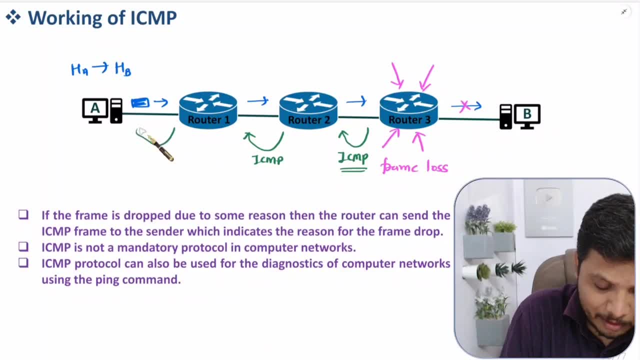 here to router one. And now router one will give ICMP frame to host A And this frame says what This frame says. this frame the transmitted frame by A that is lost somewhere in the medium, So you will have to retransmit it. 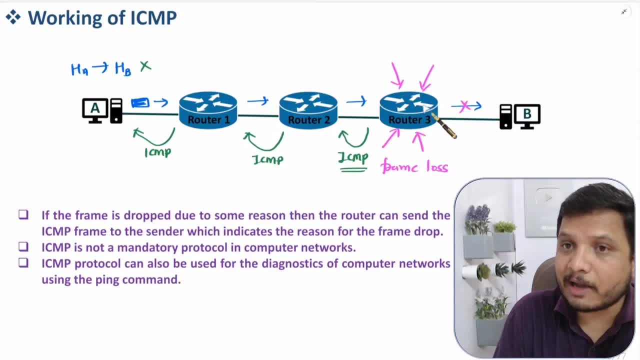 Or you can find some other path. The reason is: right now I am busy, So this router three, router three knows this frame could not be forwarded over here, So router three will be forwarding ICMP frame In ICMP frame. router three will say the reason. 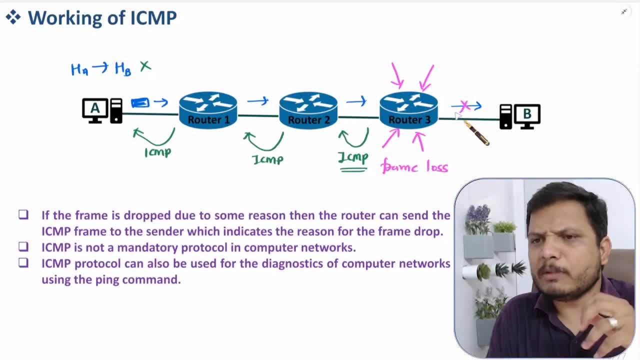 What is the reason behind this frame cannot be forwarded over here. There can be so many reasons. In next video I'll explain you applications of ICMP protocol in which you can use this Minimum: 10 to 15 reasons that I'll show you practically. 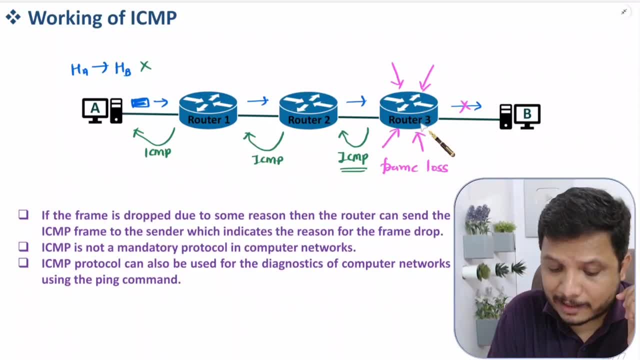 But right now consider: because of some reason, let us say, frame is lost. So by ICMP reply, this router will say: this frame is lost, You will have to transmit it to host B And you may have to choose some other route, even as if router three is very busy, right? 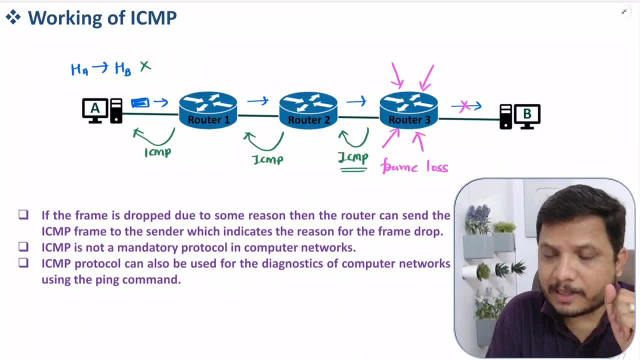 So that is how working is there. But remember this: ICMP, that is not mandatory, It is optional. Right, It is optional And by ICMP we improve reliability. Now I'm going to explain you how frame structure is there with ICMP protocol. 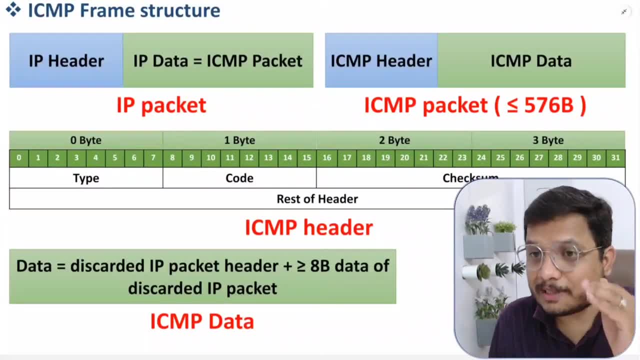 So in frame structure of ICMP, you should know ICMP that is implemented on IP. IP is internet protocol, ICMP is implemented on IP. Let me show you how See. this is IP packet, internet protocol packet, Like we have seen. IPv4, right. 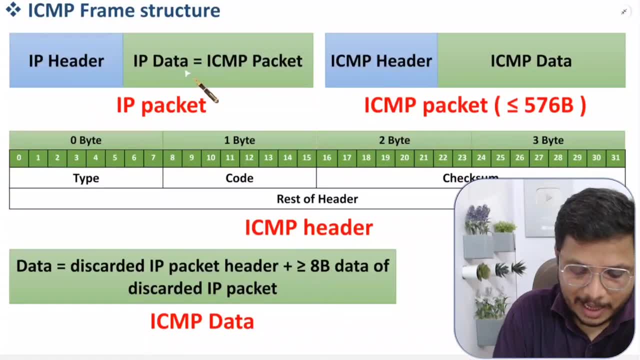 So with IPv4, we have IPv4 header and IPv4 data. So similarly, IP packet that is having IP header and IP data. Why I'm saying IP? The reason is in IP we are having two categories: IPv4 and IPv6. from saying this in general, 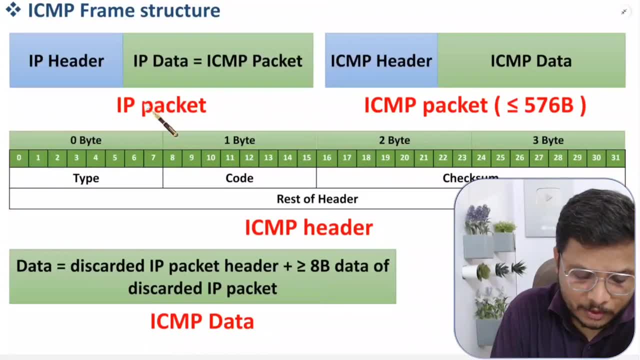 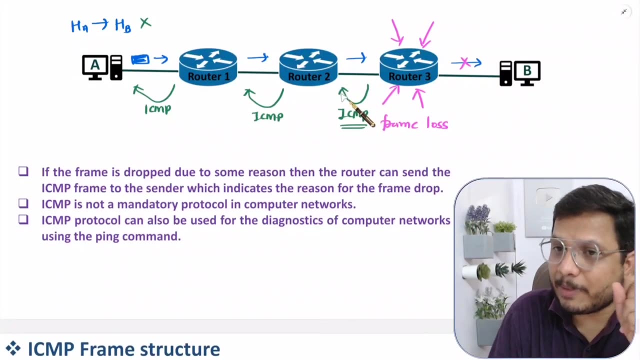 like it could be IPv4 or IPv6, right? So you see, here in IP data we are having ICMP packet. See, we are technically we are having IP packet. So whenever you forward, whenever you forward ICMP packet, at that time practically will. 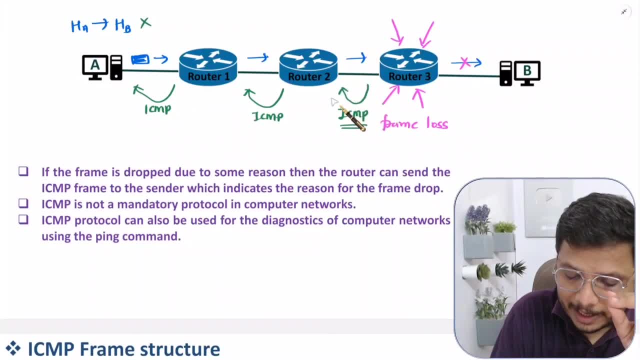 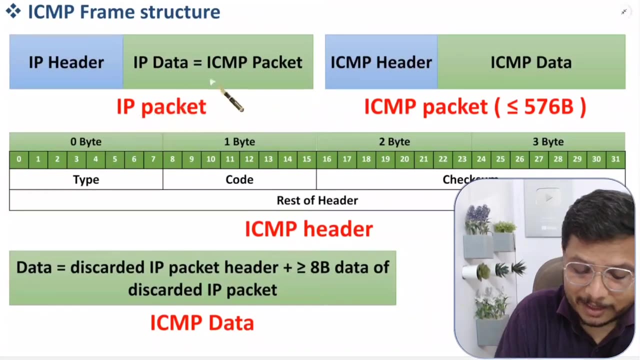 be forwarding? what IP packet only In this IP packet. in this IP packet, router 3 will give source address of router 3 and destination address of host right. That will be IP packet only, But inside IP packet, inside IP packet there will be ICMP packet. 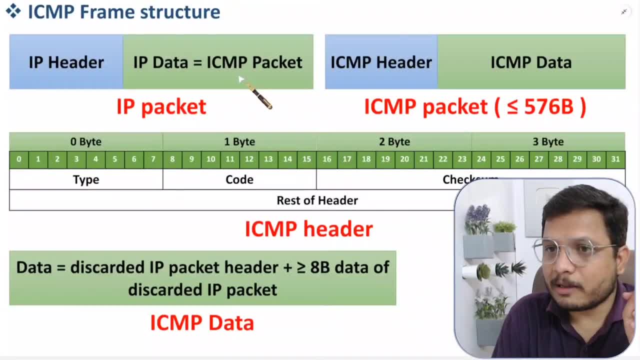 So in data part of IP There will be ICMP packet. Now what is ICMP packet? So again you see ICMP packet, that is, having ICMP header and ICMP data. Now let us try to understand. what is ICMP header right? What is ICMP header? 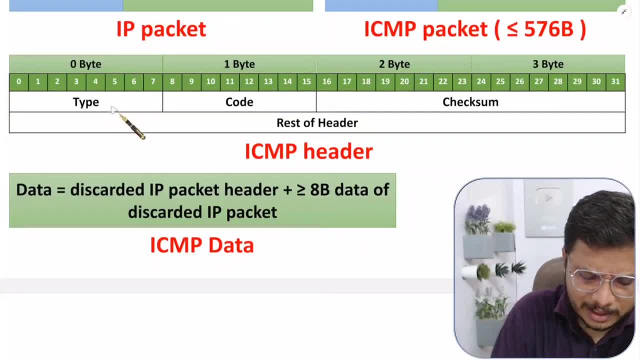 You see ICMP header that is having generally three fields only. We don't use the rest of header that is having four bytes. but we don't use this Type code and checksum. Obviously checksum is what Checksum that we use it to identify. 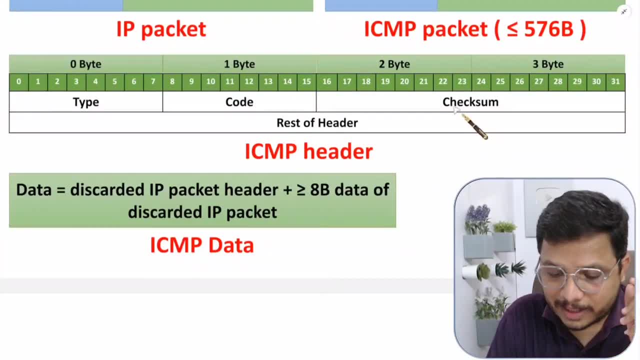 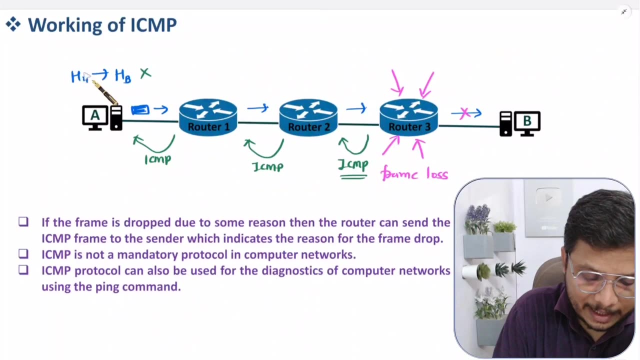 What is checksum? To identify errors? right, So checksum is used to identify errors Here. type and code. that explains you what is the reason behind frame loss. See what is happening here. You have been sending, you have been sending frame from A to B and that frame have lost. 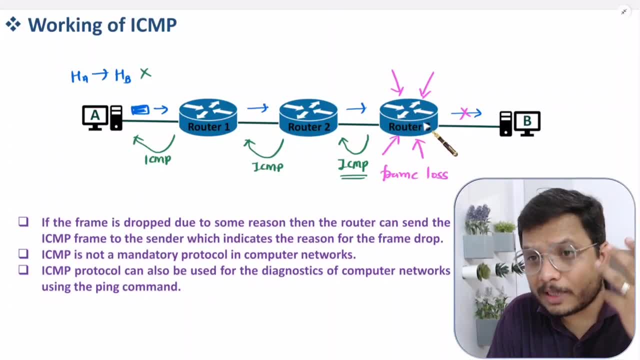 over here at router 3.. So there can be so many reasons right. There can be reason like host B, Host B is busy, Host B is busy. There can be reason like this link is this link is having failure. There can be reason like this link is having too much traffic. 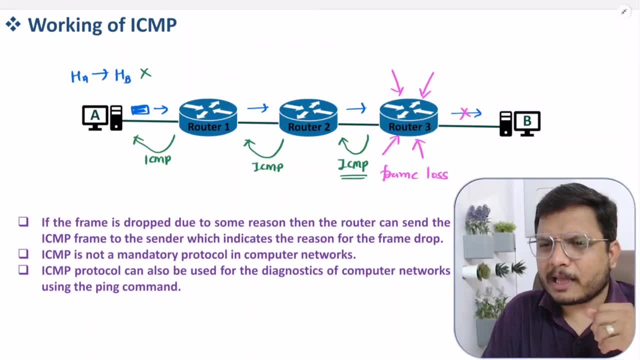 There can be reason like this router is so busy. There can be thousands of reasons, practically right. So because of some reason, because of some reason, frame is lost. So that reason, that reason, that reason can be explained by type and code. 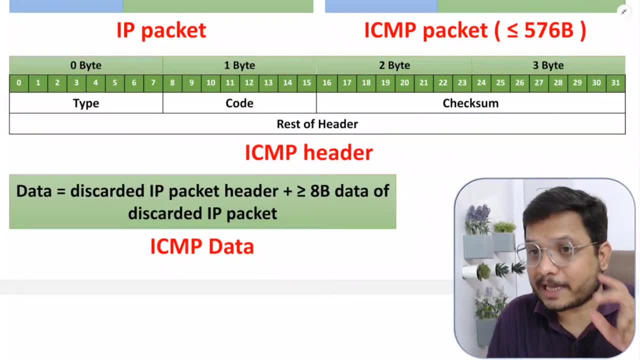 So that is the reason. right, Type and code field. So in application part in next video I'll explain you applications of ICMP, in which I'll explain you varieties of reasons why frame may get lost, right? So right now, just consider type and code field. that explains you the reason behind frame. 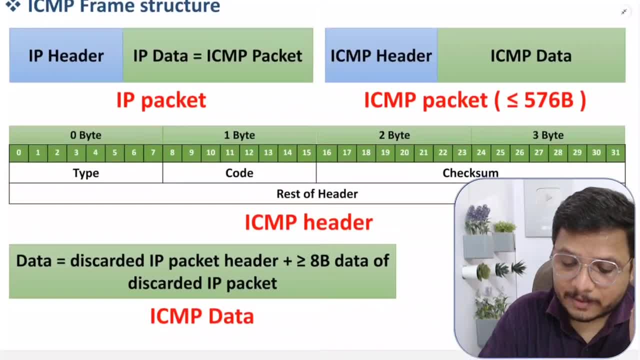 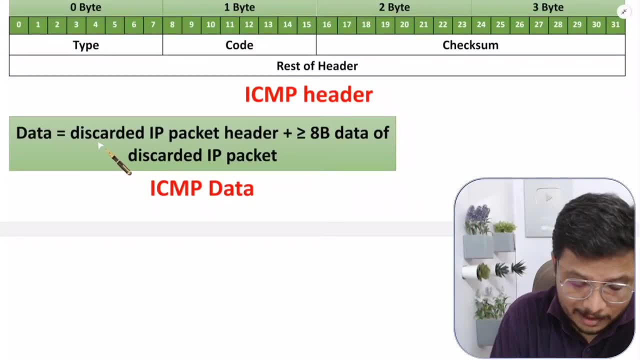 loss. Now very interesting part that comes. that is, ICMP data. Now, what is ICMP data? You see, See, this data will be discarded. And what is ICMP data? Discarded IP packet header plus greater than 8 bytes of data of discarded IP packet. 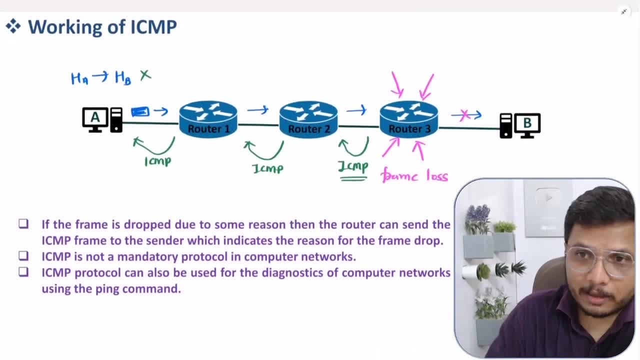 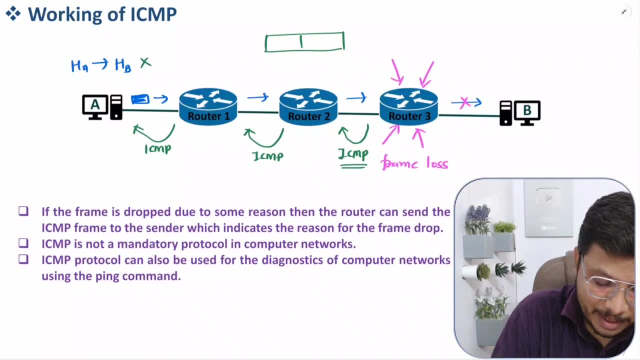 Like. you see what is happening here. Here we are forwarding, Here we are forwarding one frame, So obviously this frame will be having how many information. This frame will be having header right And this frame will be having data And this is what IP frame right. 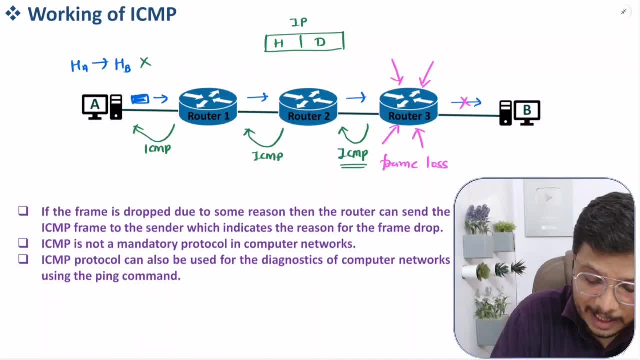 This is what IP frame. So when this frame, When this frame, When this frame is getting lost at that time in data field, how many things that, how many things that will be there. See this header and greater than some portion of data that will be there. 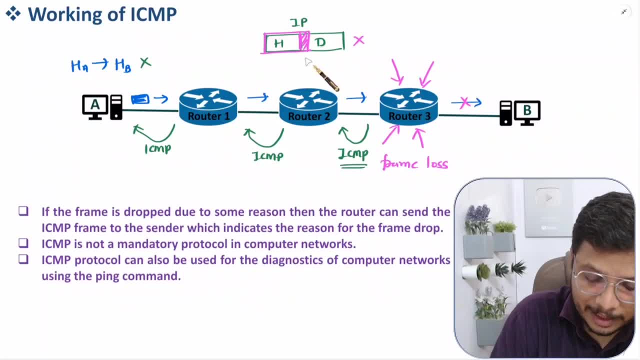 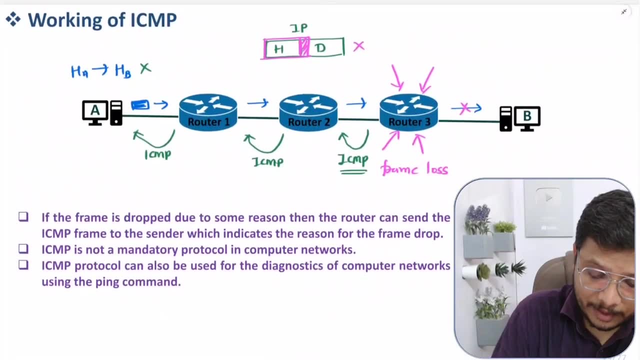 Some portion of data that will be there, right, And this should be greater than 8 bytes. This should be greater than 8 bytes, right? So here the frame, the frame which is getting lost, That header, That header Plus. 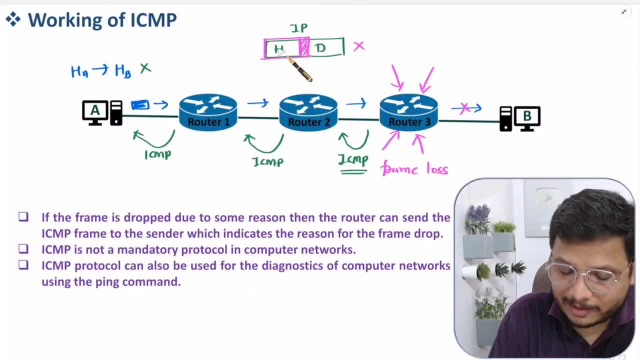 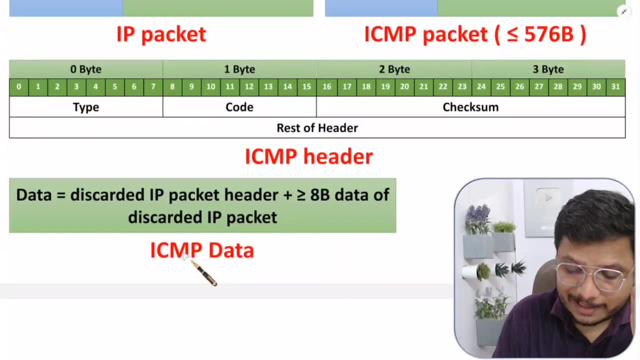 That header Plus More than 8 bytes of data. That header plus more than 8 bytes of data portion. right, That we are adding, That we are adding in ICMP data. So ICMP packet That is a combination of ICMP header and ICMP data.